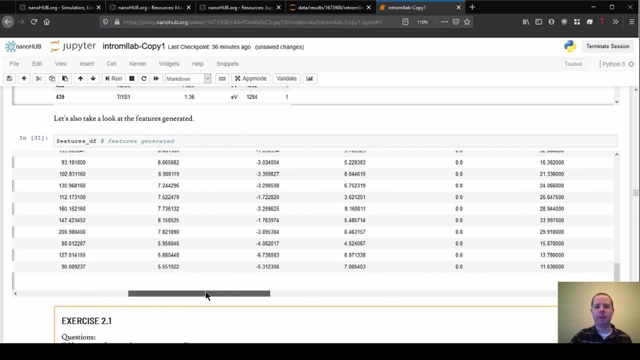 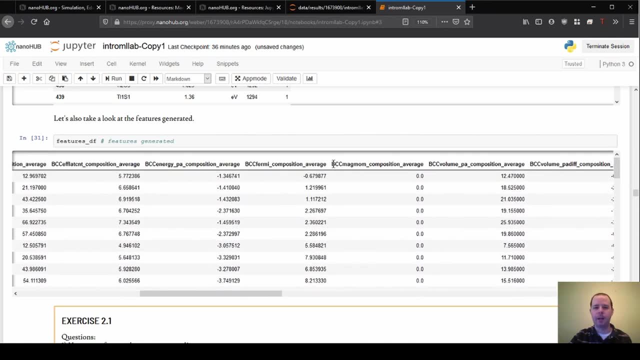 when we looked at the features here in our data frame, what we might notice is that some of these are the same. So look at this column here, right here, that I'm going to hide, So I'm going to highlight. so this is BCC magmom composition average. This is a magnetic property of the 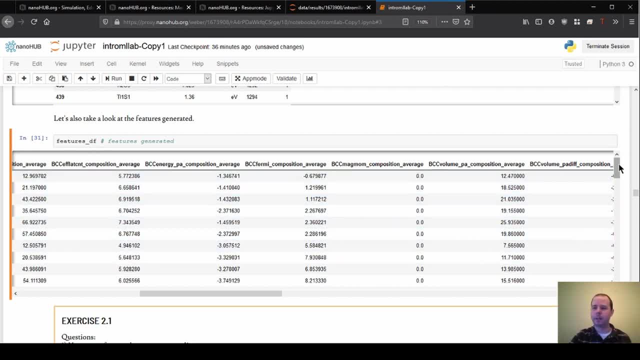 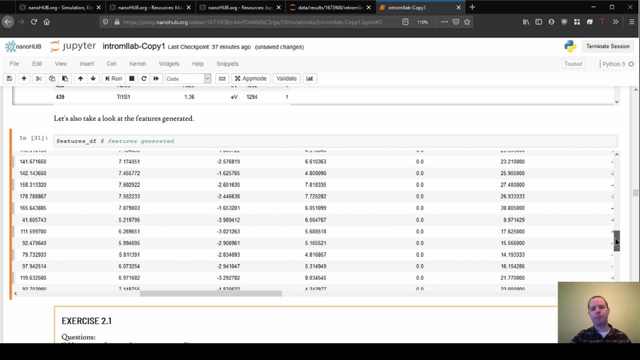 materials, and all of these are zero as far as I can tell. So let's scroll down here and look briefly. We're skipping some of the section again. we have a bunch of rows here, so we're not going to output all of it, but for all the rows that we're looking at here, all of these are zero. 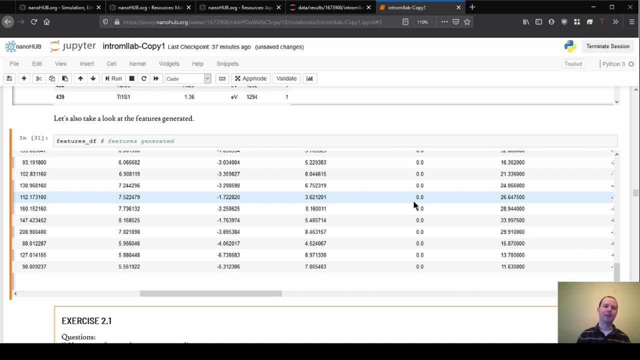 So this is basically a useless feature as far as we can tell, and if we gave this to the model, it would basically give us no new information. So the first thing that we're going to do for this is we're going to remove all of these columns. So we generated a huge range of them. 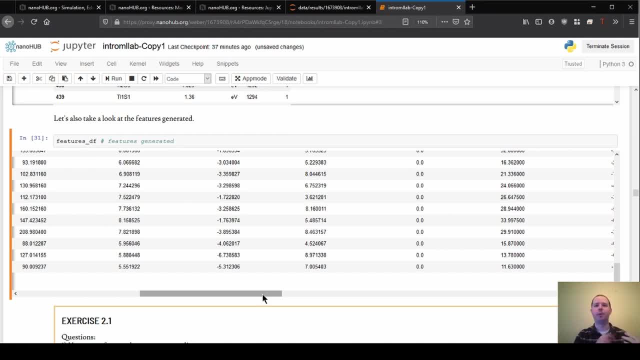 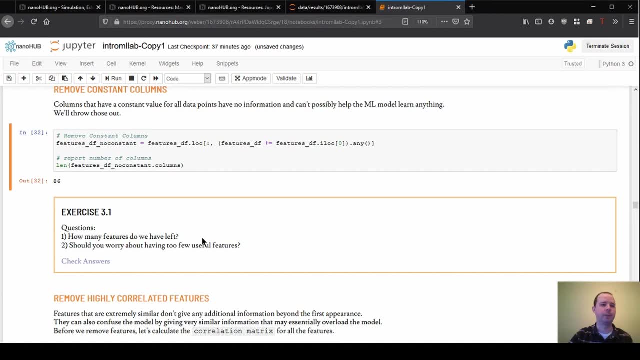 basically, you know automatically, and now we're going to go back and try to remove the ones that we don't think are useful. So the first ones we don't think are useful again are the constant ones. So we can just do this simple filtering step here where we say: you know if something. 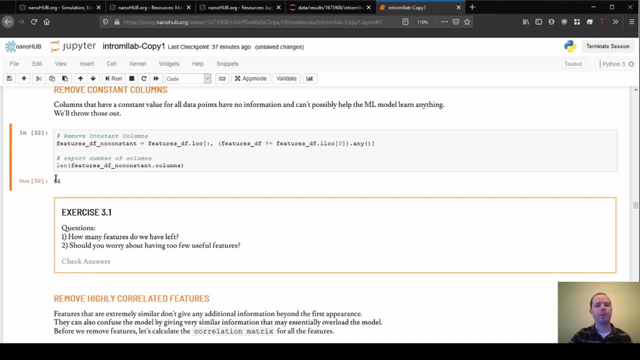 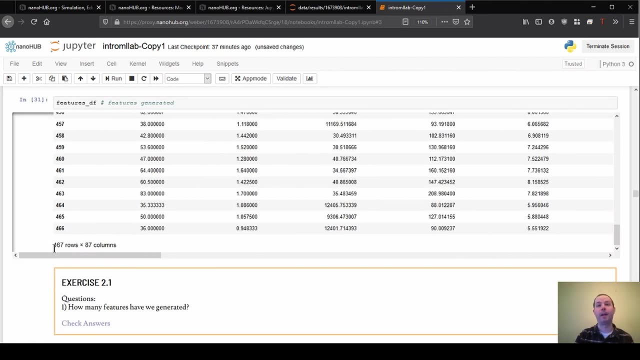 isn't changing at all. let's just take it out, And each time we're going to output the length of our column set here. So now we're. it looks like we have 86 features, whereas previously- let's scroll back up and check- if we look at the size here, we had 87. So it looks like we only had. 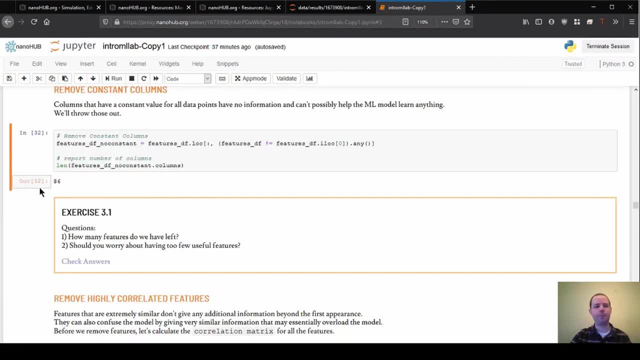 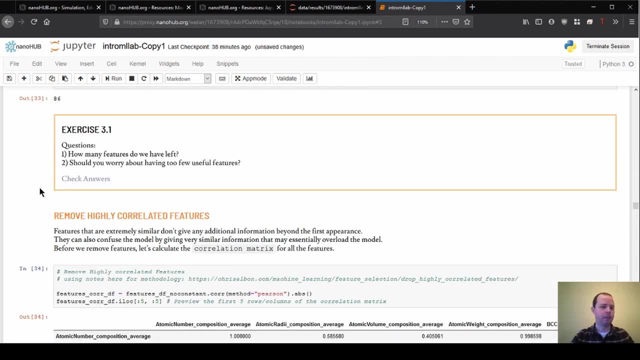 one constant column there, and it was that one that we found. So we can remove that. make sure we're not, you know, giving it any stuff that isn't useful there. And now we can move on to the next. So the next thing that we're going to do is remove something called correlated features. 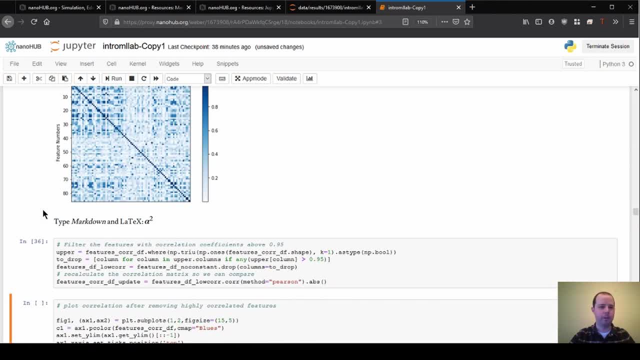 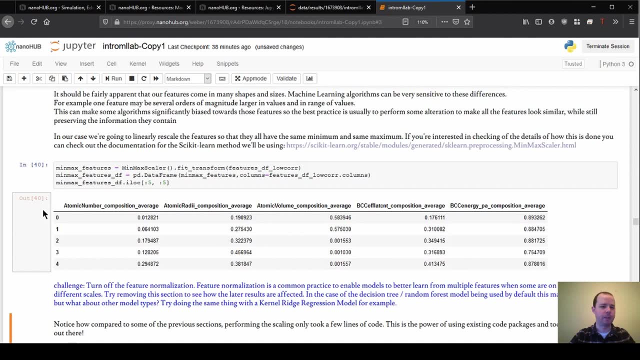 So I just executed a bunch of cells here just so I could have the output to talk through, and I think I'll go through and do that all the way to the end of the section, just so we can look at the outputs together instead of running through and having them all pop up one by one. 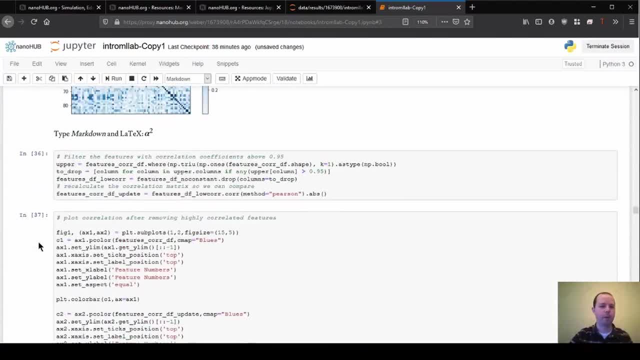 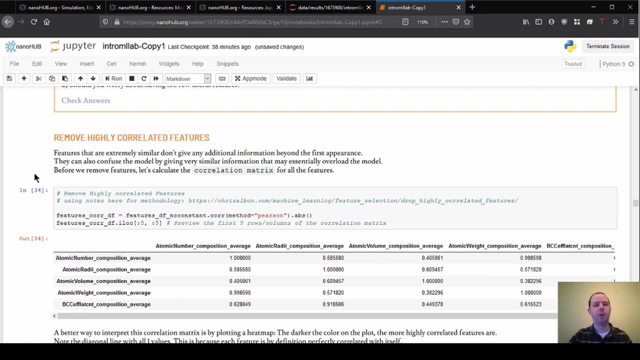 So I'm going to run through everything down to section four and I'll scroll back up and we'll talk through the outputs. So the next thing we're doing is we are removing highly correlated features. So when we talk about correlation between features, we're talking 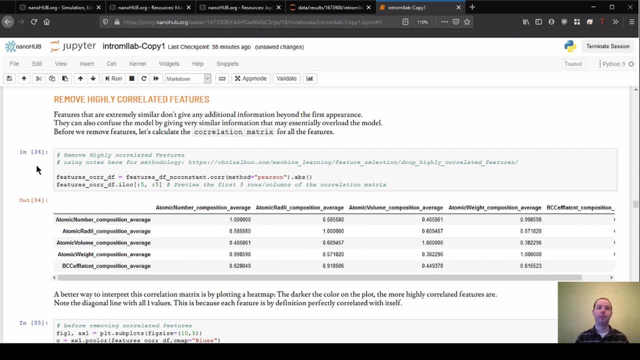 about features that are giving the same information to the model. So previously we said we identified, you know, features that don't give any information to the model. and now we're going to say what if we have two features but they're telling model the exact same information? That would be another way that we'd have kind of a useless 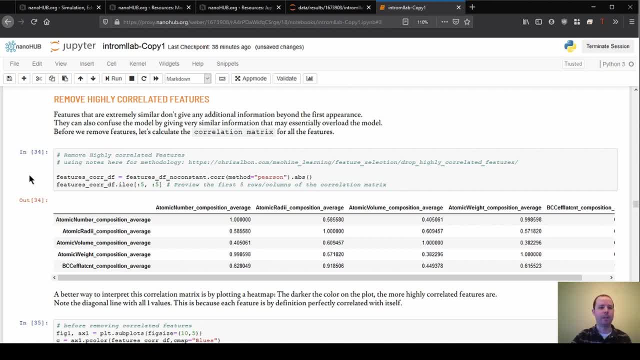 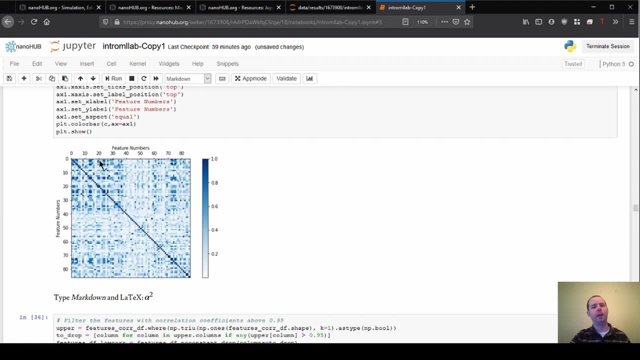 or feature. that's probably just giving noise to the model and not really giving anything interesting. So one way we can visualize the correlation and see it a little more directly is by making something called a correlation matrix, which is shown here. So what we're showing is the numbers of the features on each axis and then we're showing how well correlated 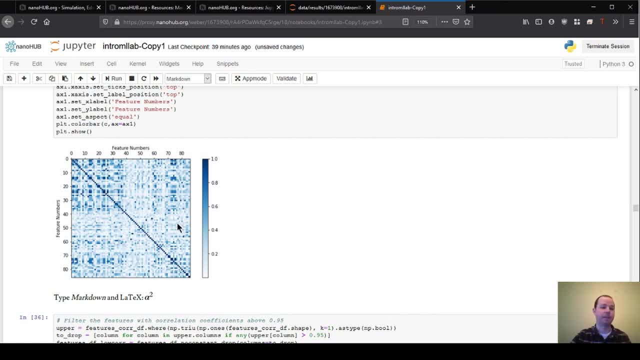 they all are with each other as intensities here. So what you can see is there's this diagonal line and this is showing that you know everything is perfectly correlated with itself. That means you know everything is exactly the same as itself. So the higher the color, the the closer they are to. 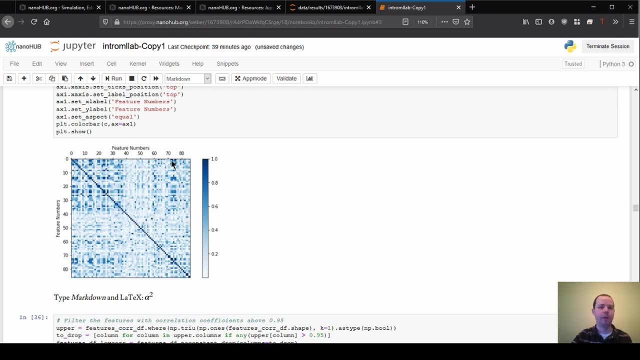 each other. So what we see is that there's some here that are very dark blue. There's this kind of pocket in the in the top right here, around 70, between 70 and 80. So there's definitely features here that are they're very highly correlated with each other, which means they're just not giving any. 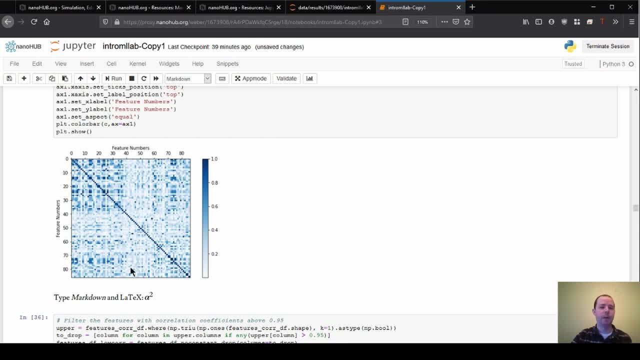 additional noise to the model. So what we're seeing here is that there's some here that are very highly correlated with each other, which means they're just not giving any additional information, And then there's other ones that are, you know, very close to white, which is not correlated with. 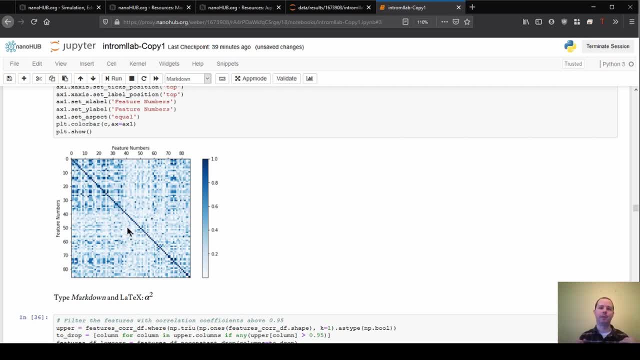 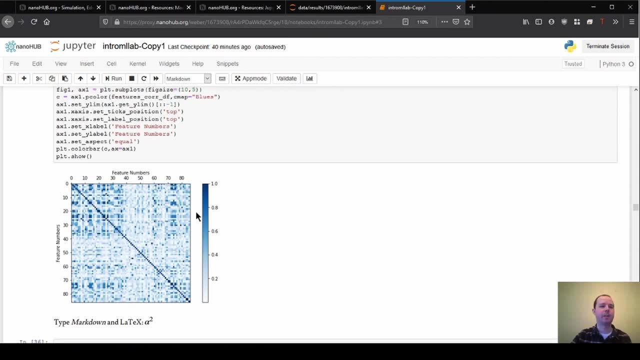 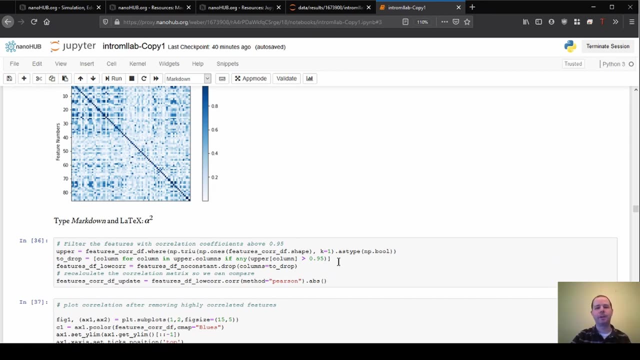 each other at all, which means they have totally separate information, which means, hopefully, they're giving again different information to the model and allowing it to learn things from all that different information. So what the cell blocks do here is they basically calculate this huge correlation matrix and then what we're going to do is we're going to filter everything that's. 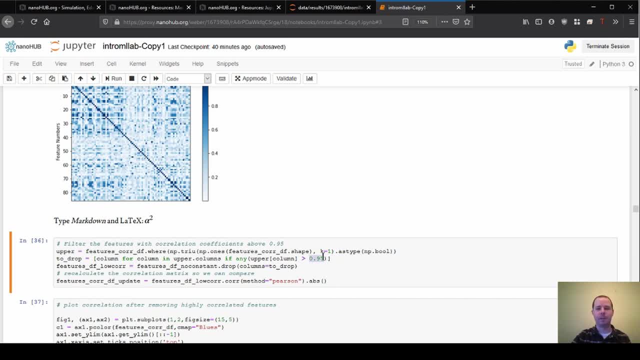 above 0.95.. You can see this here correlated with each other. You can filter above that and we'll say those are, you know, too highly correlated. This is somewhat of a subjective cutoff here, so it's not set in stone that that's like the right cutoff that we should make. That's. 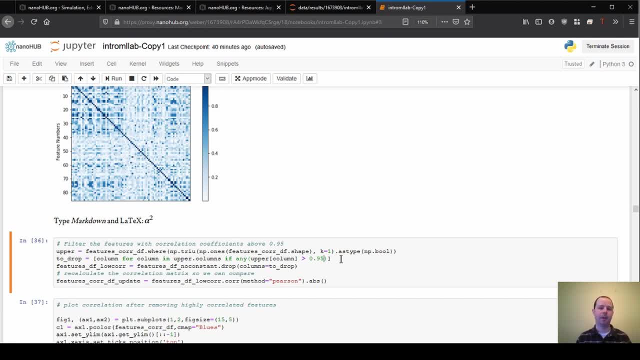 a choice that we can make as we go along. So if you're following along at home, you can definitely change this and see how it affects your results. So this is one way you can sort of change things. Just know that you know the lower you set this value, the less features you're going to have. 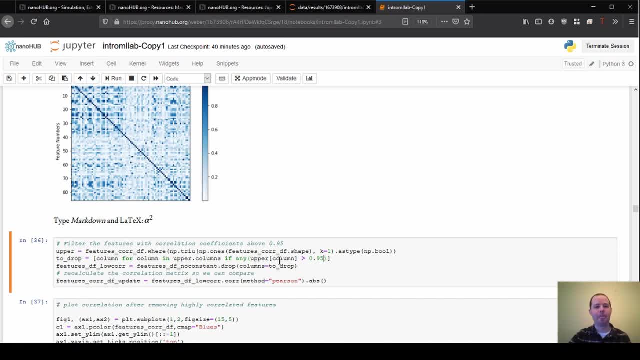 going forward, but maybe the better features you're going to have. So that's one again decision you can make, and it'd be interesting to see you know what results you're going to get, What results you get if you're changing those. For now I'll just leave it as it is. 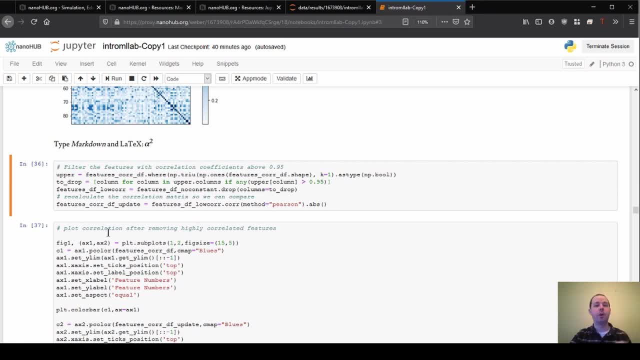 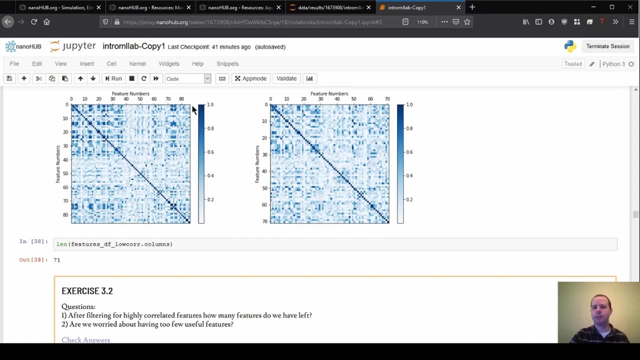 and we can potentially come back later and start looking at it more. So once we make that filtering step, we can re-plot and look again and what we see is that previously again, we had, I think, 86 features, if I remember right, and now, with the plot on the right. this is after we've done the filtering. 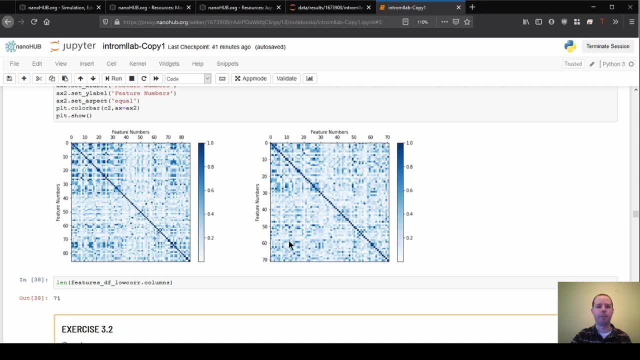 step. Now we're down to 71 features and we can see that reflected in the numbers here. So overall, when we look at the plot now, we still see the diagonal line because everything's correlated with itself, But now everything is cut off below 0.95, so there's none of those super, super dark. 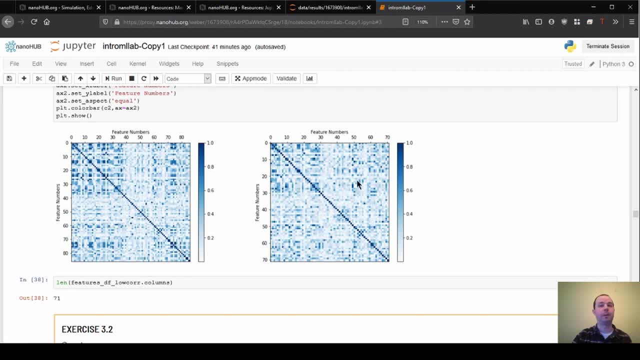 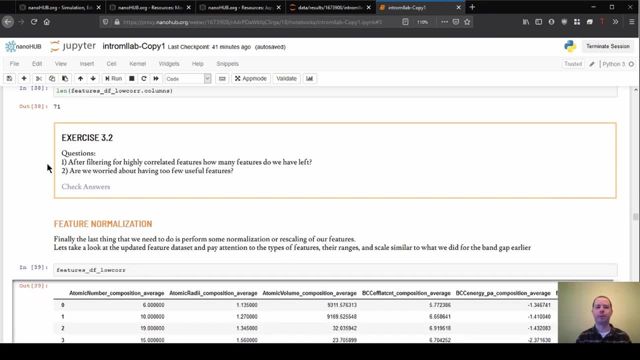 values that we had previously, although you can still see there's some that are, you know, fairly up there. so if we lowered down, we would definitely keep filtering some of these. So that's the second step that we're going through for doing our filtering step, and the last, or our feature engineering step, I should say 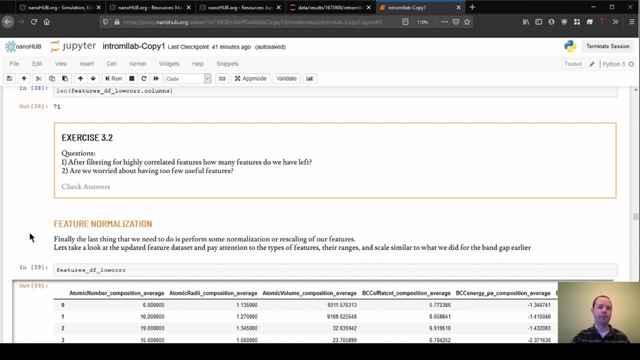 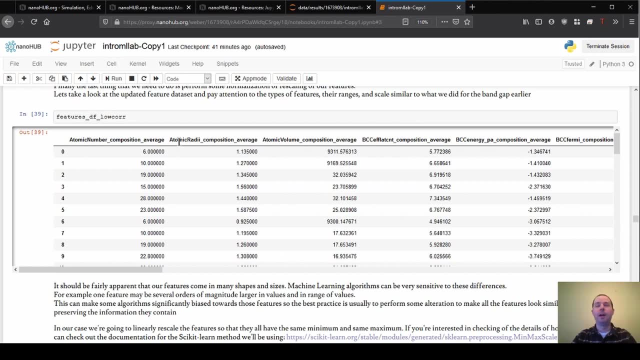 And the last thing that we're going to do is something called normalizing the features. So what you might have noticed previously, and I think what we're showing here in this output, is features are very, not only different in the information that they're giving from each other. 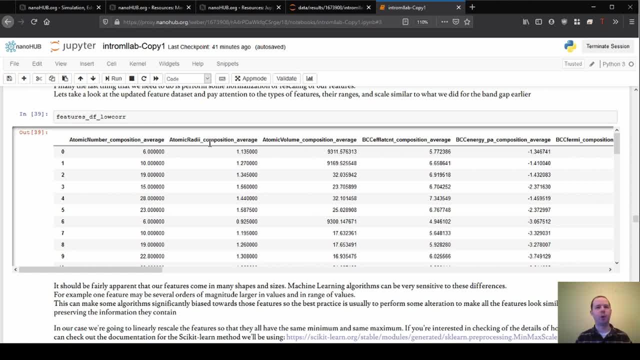 they're also just different in the kind of scope of values themselves. So if I call attention to these two columns in particular, the atomic volume and the atomic radii, what we can see is that atomic radii are generally on the scale of one or so, it's 1.1, 0.9, 1.2.. They probably, you know. 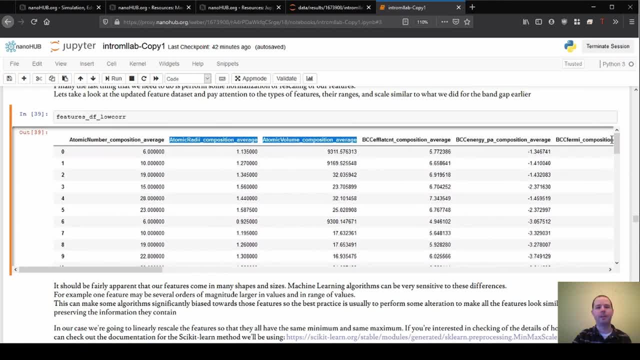 they can get up to a little larger, a little smaller than that. but on this, if you looked at the range of features, they definitely don't go above, you know, 10 or 20 or something like that, Whereas the atomic volume here is in the thousands. it's, you know, 9000 here, 9000. 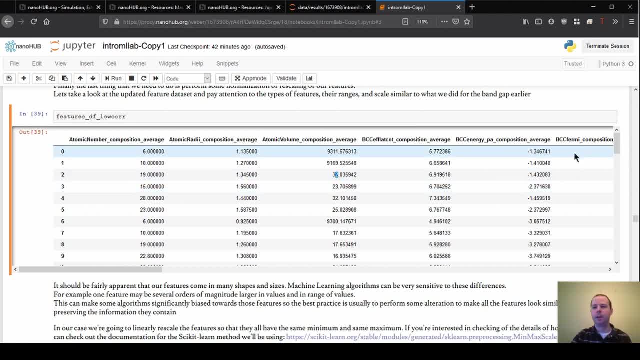 this one's 30, so this has a huge range on it, going from single digits up to 12,000 in this case, And what this means is that if we give both of these features to the atomic radii and the atomic radii- and the atomic radii of the atomic radii of the atomic 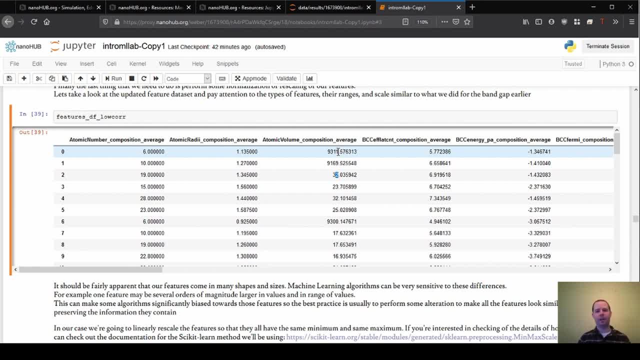 the model. this is especially important depending on the model type that we're using, but again, this is just a general good practice. if we're giving these to the model, what can happen is that the features that are just larger than the other ones or have more variation in them can end up. 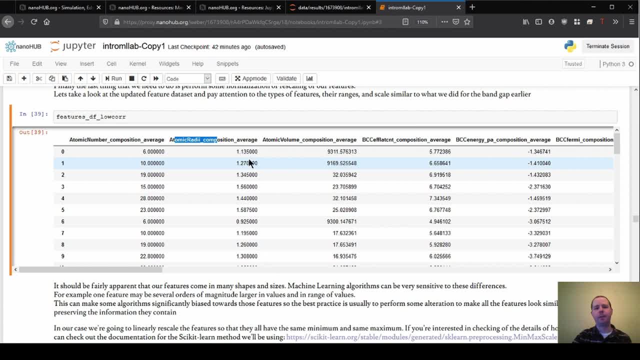 dominating the model. so even if atomic radii was really important, the fact that it only ranges from, potentially, you know, 0.9 to 1.2, 1.3, 1.5 means that it might get kind of swamped out by something. 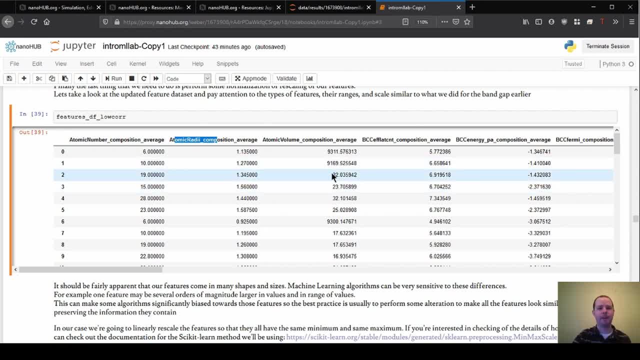 that's varying from 30 up to, you know, 9 000, something like that. so what we're going to do is a process called normalization, where we just take the range of the features and we shrink them down so they're all on the same scale with each other, and what we can see when we do that here. 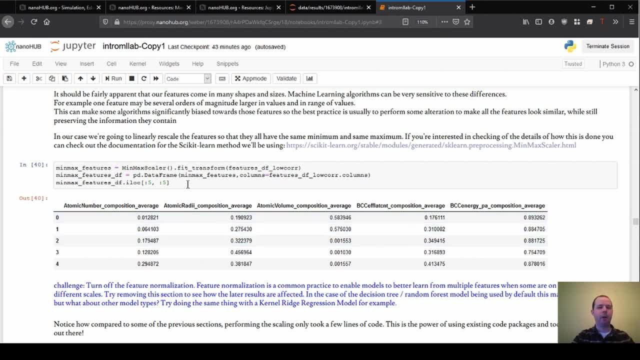 in cell number 40 is that now we have all of these scaled so that they range from 0.9 to 1.2, 1.3, 1.5 means that it might get kind of swamped out by something that's ranging between the same values. in this case i think we chose a process here called min max. 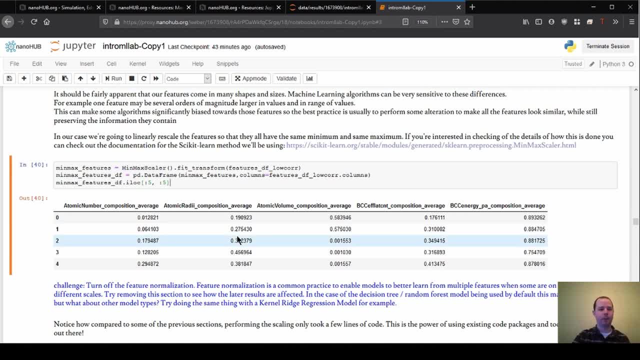 scalar, which sets the range from 0 to 1, so everything now has a minimum of 0 and a maximum of 1, and what this means is that now they're on the same scale with each other, but all the information there should still be intact. we haven't done anything to scramble up the information we've. 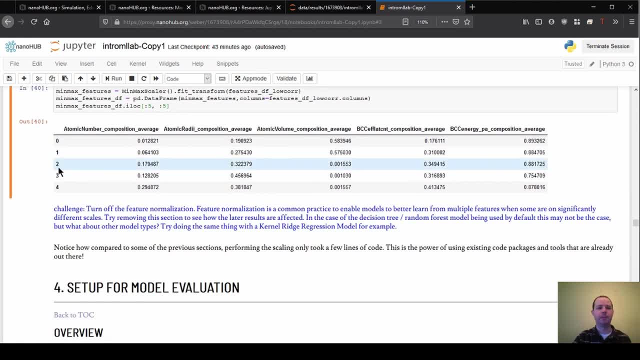 just kind of compressed the range that it can be expressed in. so now, if we feed these all into a machine learning model, hopefully one of them won't get weighted above the other just because its values are larger than the other. so again, this is a very common practice. there's a 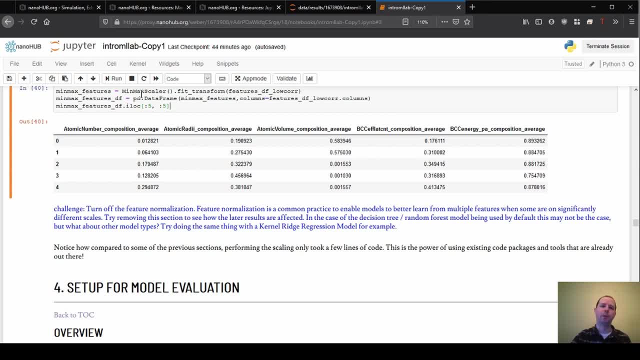 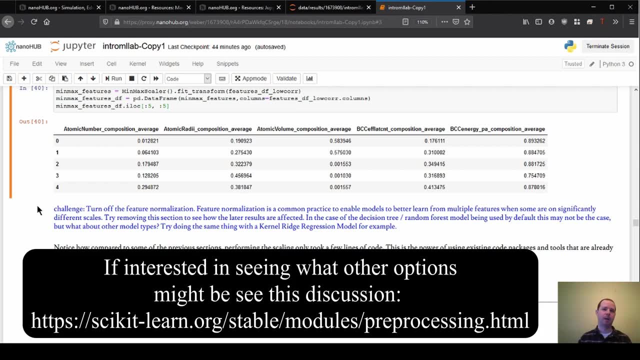 few different ways to do this. this min max scalar is just one way we can do that and that gets us through the feature engineering steps. those three fairly basic things we can do. they're definitely much more complex and specific things we can do depending on more targeted applications or 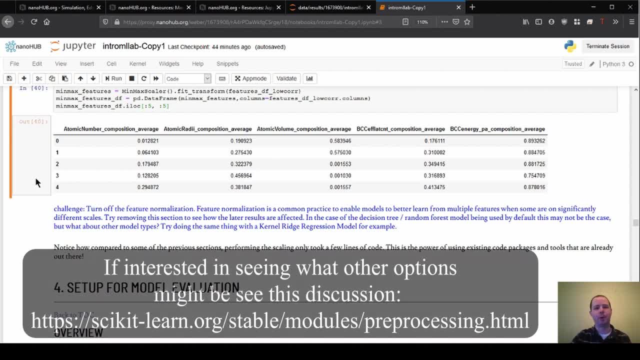 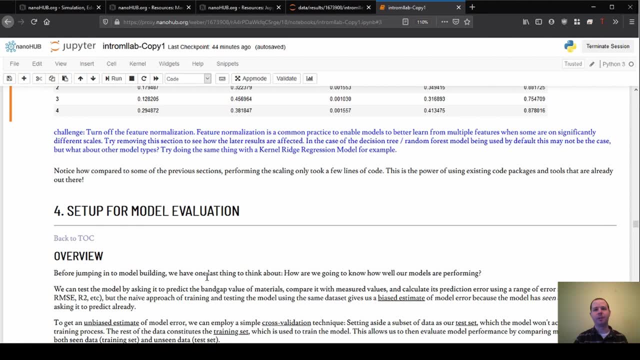 depending on the specific project that we might be working with. but this is the idea of feature engineering as a whole. so next time we'll dive in for section four, which is on model evaluation. we'll start to talk through, you know, how do we actually assess a model, and then we'll hopefully start, you know.